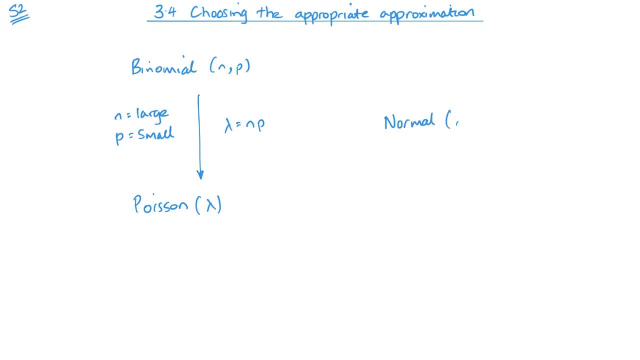 here. I quite like the way it's done in a few of the textbooks, So I'm going to keep a similar method. So here now, if n is again large, so we can go this way: n is large This time. p has to be close to a half. 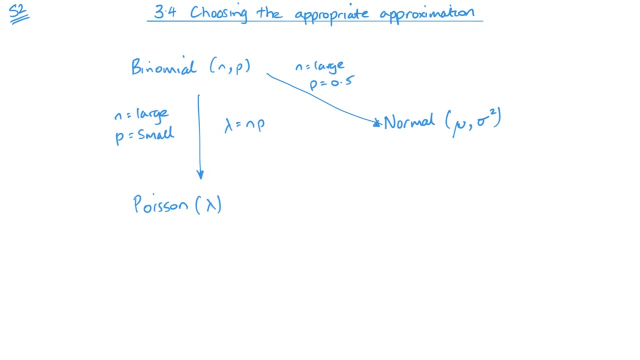 So here you can see really the difference between the two. You know, when you're looking at approximation, it's whether p is small or p is close to one half. Now, again, that's not always helpful. So what I would say is, when you're doing this kind of approximation, 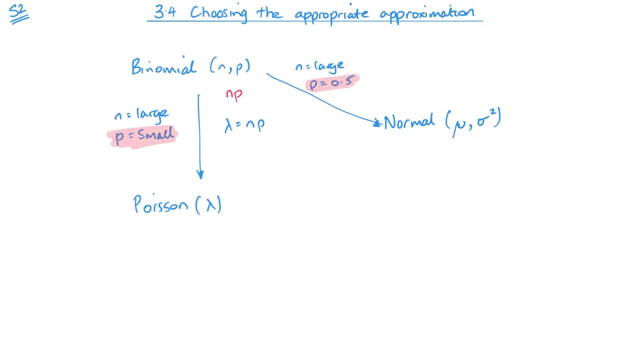 work out np, which is your mean for both. And if this is less than or equal to 10, then you should be able to use Poisson, And if it's greater than 10, then you would use the normal, And that's a good way of checking it. So that's the binomial done with, So starting, 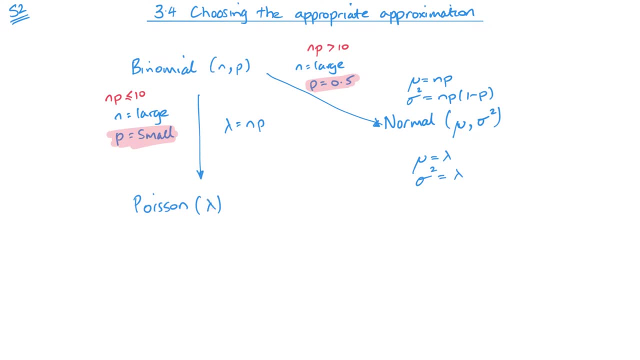 with binomial. we can go to Poisson, As we said, or normal. So remember the only difference is p, but that can also be a little bit confusing sometimes. So, as they said, multiply them together for np less than or equal to 10. 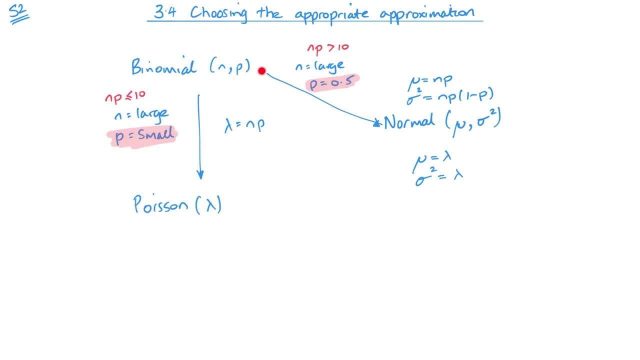 should be Poisson Greater than 10 should be binomial. Now for Poisson. our only option is a normal approximation. here is that our lambda is large. you'll notice in the tables lambda only goes up to 10 and all questions you should be able to do with the tables, not just with your calculator. 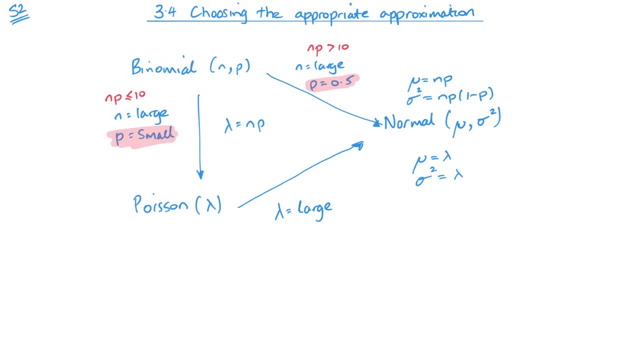 so you know, if you get a value of lambda that is greater than 10 within the question, then it is implying that you're doing a normal approximation there. so that's. you know that. one's quite straightforward. if you've got a Poisson question and it asks you to use an appropriate 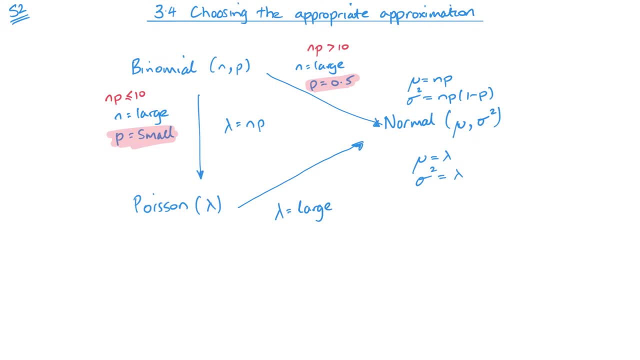 approximation. well, your only option is normal. now there's a little bit more than just that. so, as we talked about before, binomial and Poisson is discrete data, so if I'm changing between binomial and Poisson following this line, then I don't need to worry. 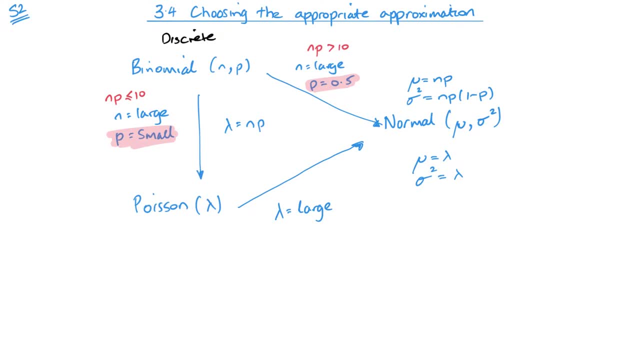 about anything, but if I'm approximating either binomial or Poisson with the normal distribution, and the normal distribution is continuous data as net, which means that we need to use continuity correction. so when you go from either of these two to the normal, we need to use continuity correction. and a nice way. they show that in a lot of the text. 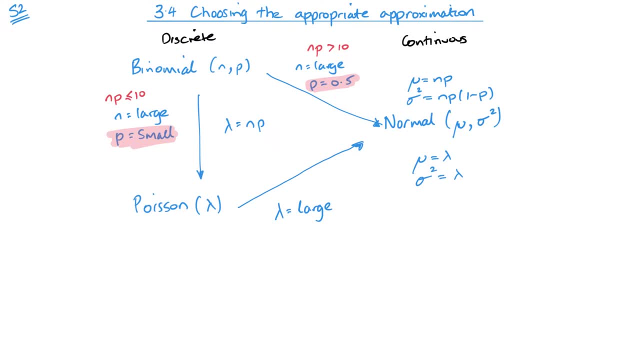 books and online is just with a simple line which I'll pop in now and there we have it: cross the line and you need to then use continuity correction. okay, remember when you are doing that, just same as, like I always say, to avoid making mistakes, change everything to a less than or equal to, or. 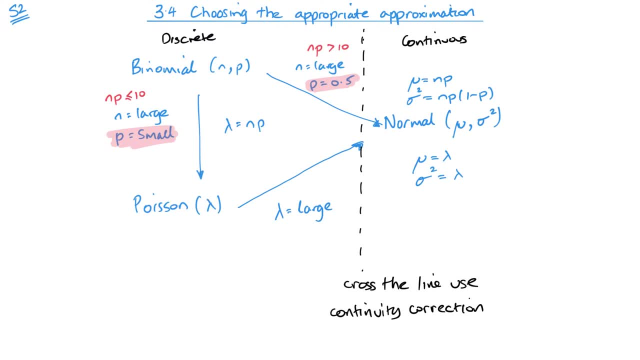 greater than or equal to first, and then do your adjustment that way, that consistency. doing it that way in every question will mean that you'll start doing it almost without thinking and you're less likely to make those mistakes than if you try changing from a greater than or a less than. 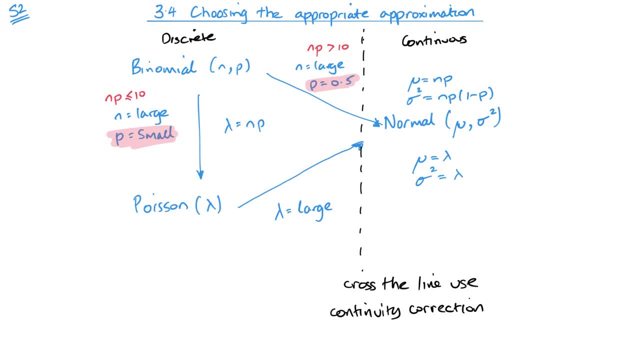 mixed in with less than equal to and greater than equal to. so I think the best thing to do here is to look at some exam questions. what I'm gonna do is I'm not gonna do any examples on this video. what I'm actually gonna do here is this: just we're gonna go to email and cand Bible- some key injection- and so what I'm gonna do is I'm not gonna make any equation and I'm just gonna take results from and roughly get a score. they're pretty much the samejalicab and my answers are all there's that we can get over here. you can take them with the final unit of 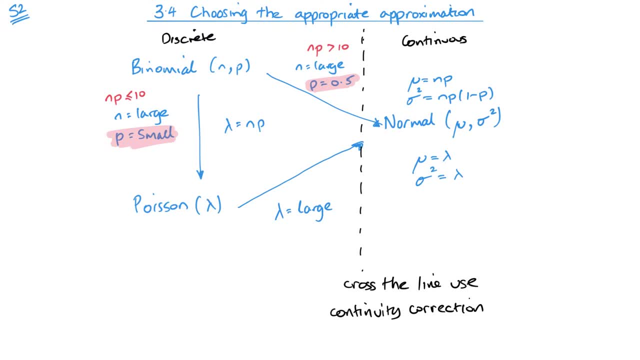 any examples on this video. what i'm actually going to do is i'm going to do a question and then the answer, the work through question, work through question, work through. that way then you can have pause the video, have a go the question, mark it before moving on to the next question. 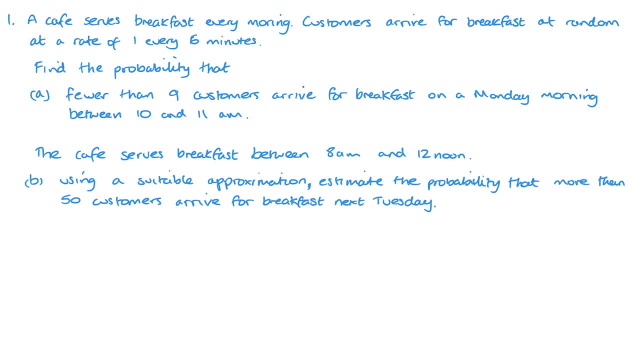 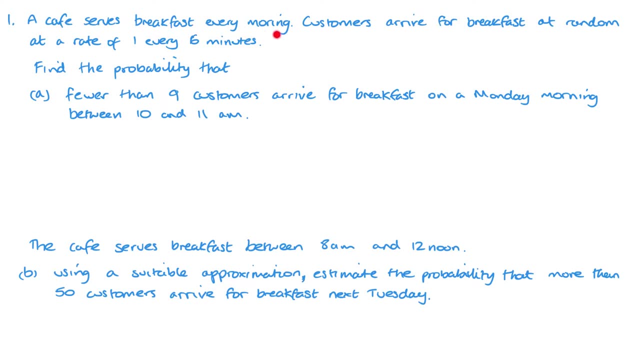 so here we can see a cafe says breakfast. every morning customers arrive breakfast at random at a rate. so there we have that word rate, seeing that we pretty much confirm that this is poisson and we can see the rate is, and we have a question mark. and we have a question mark. 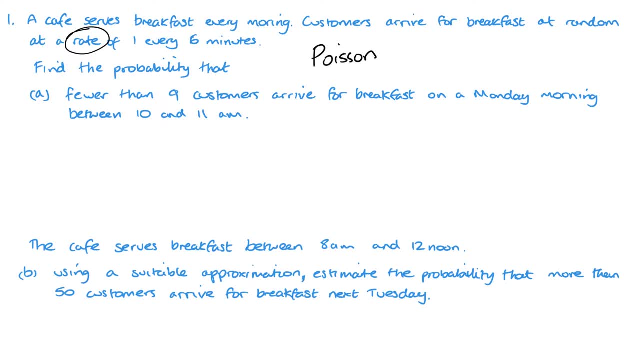 every six minutes. now for a we've got between 10 and 11 am, so that's one hour, isn't it 60 minutes? so we think one every six minutes. so in 60 minutes there will be 10, so my lambda is 10. so we're looking at our distribution as follows: 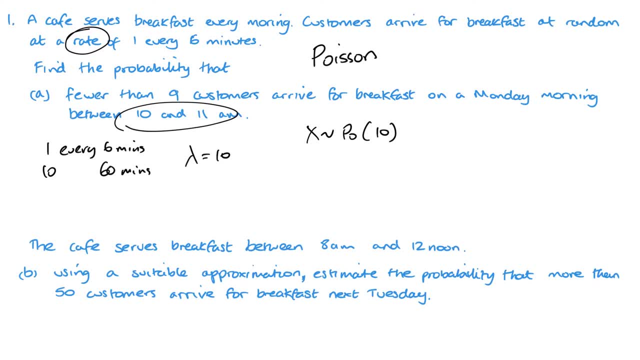 X is distributed using Poisson, where our parameter is 10. so we want to find fewer than 9. so we're looking at the probability that X is less than 9, and that's the probability that X is less than or equal to 8. so this should be. 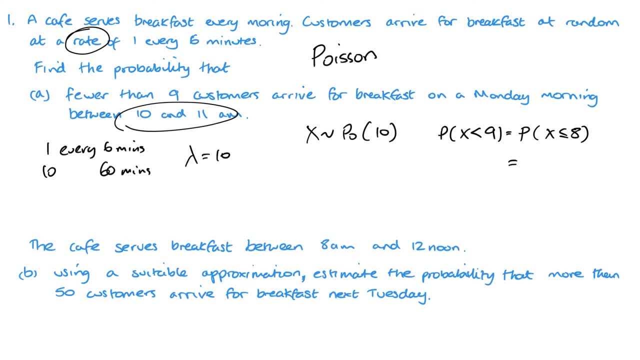 nice and easy, very straightforward one. less than equal to 8, value of lambda is 10. we can look this straight forward. and then we can look at our distribution as straight up in our tables, and here we can see it is 0.33 to 8. now moving on to 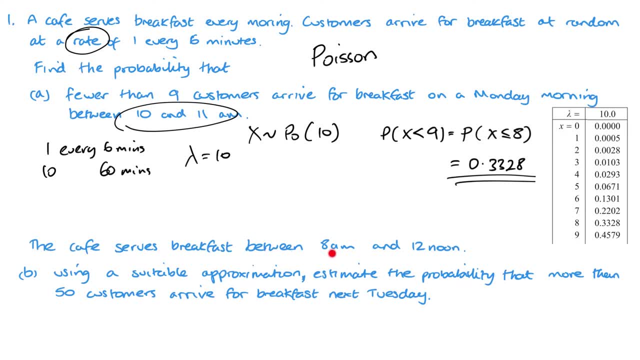 the second part, we can see the cafe serves breakfast between 8 am and 12 noon, so that's going to be four hours, isn't it okay? so value of lambda for one hour was 10, so for four hours it's going to be 40. 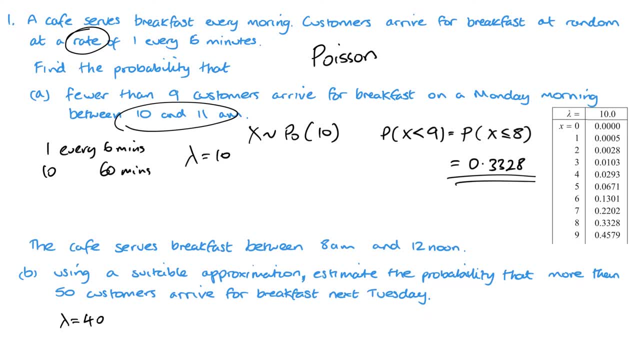 isn't it? so we've increased that value of lambda. lambda is now large, so it should be an approximation and, as you can see here, using a suitable approximation, estimate the probability that more than 50 customers arrive for breakfast next Tuesday. now, luckily for s2, we only have to think: well, we've got Poisson has to. 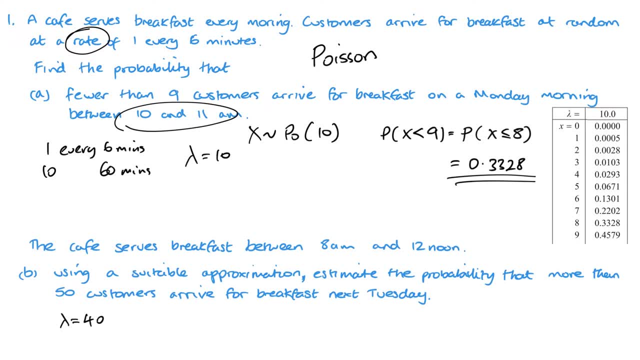 be approximated with normal. okay, and we do know that because lambda is large. so this is going to give me that Y, for normal is going to be 40 and 40. if you remember, our mean and our variance are the same and what we're trying to. 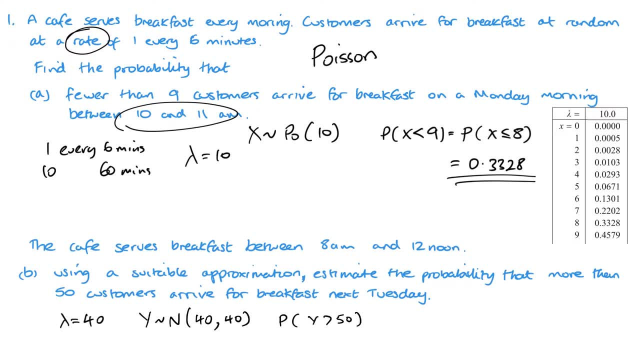 find, is when Y is greater than 50. I suppose technically it might be 50. S is greater than 50. initially, um, let's write it that way around, because I think that's a little bit better. there we are, so what that would mean in terms of our Y. well, before I get to our Y, I'd always 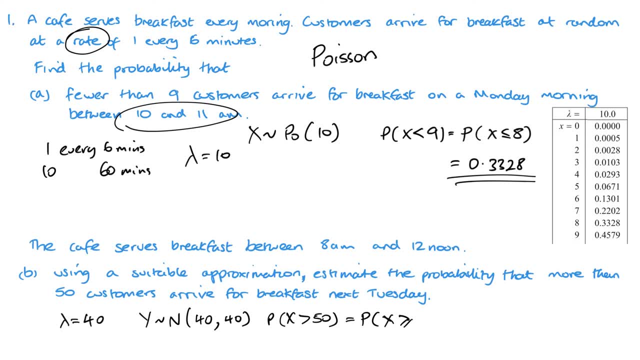 want to make it a greater than or equal to, so if it's greater than 50, has to be 51 and above, And that means then, in terms of my approximation for y, this is going to be greater than 50.5,, isn't it? 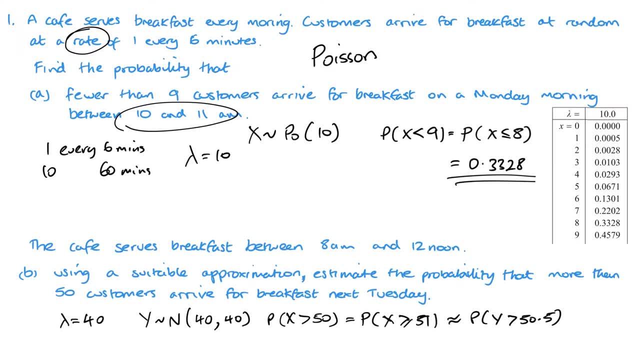 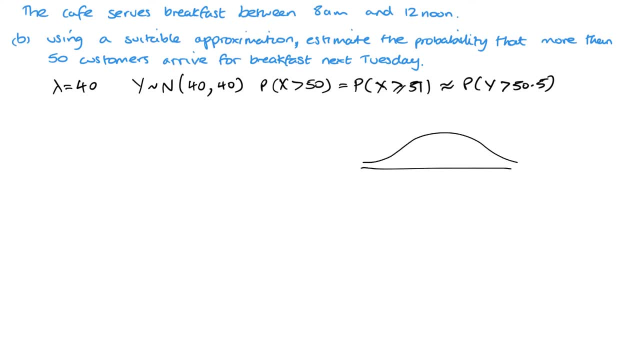 So I've got that all set up. Let's just make a little bit more room Now that we know what we're doing. I also usually like to do a sketch, Especially if I'm in an exam, you know. it just helps me think the question through clearly. 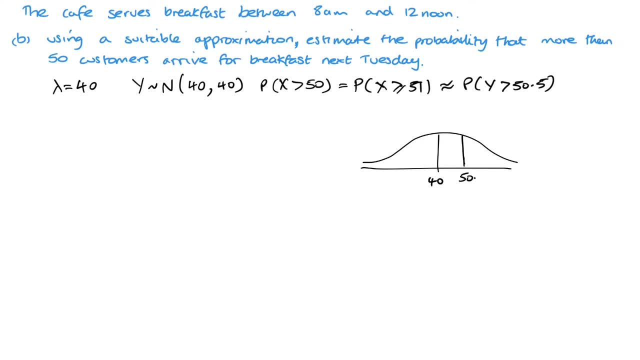 So we know our mean is 40,, we've got 50.5, and we're looking at greater than. So now we can see that it's actually a 1 minus, isn't it? So this is going to be then. you know, if I carry this on down here, this is going to be equal to 1 minus y, being less than 50.5.. 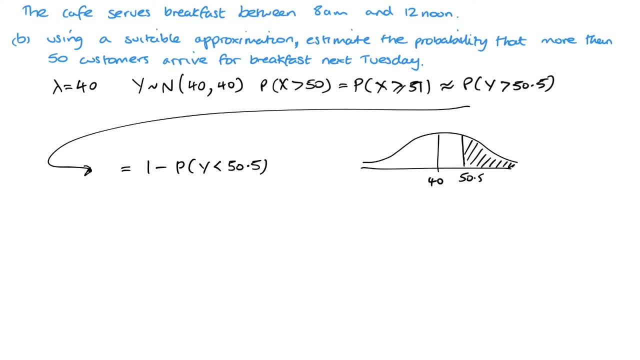 Remember, with normal, it doesn't matter if I have an equals or not an equals. This is going to be the same as with my inequality, because it's continuous data. So now I've got that, I need to turn it in terms of z. 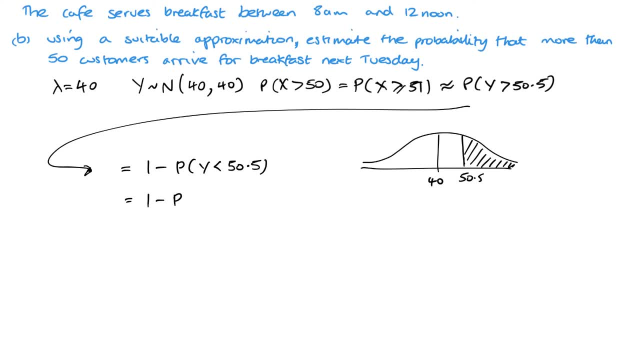 So I can do that within the question or I can do it separately. I do often like to do this separately. I just find it a little bit easier that way, So let's just pop this up ready. So over here we've got our 50.5 minus 40 over the square root of 40.. 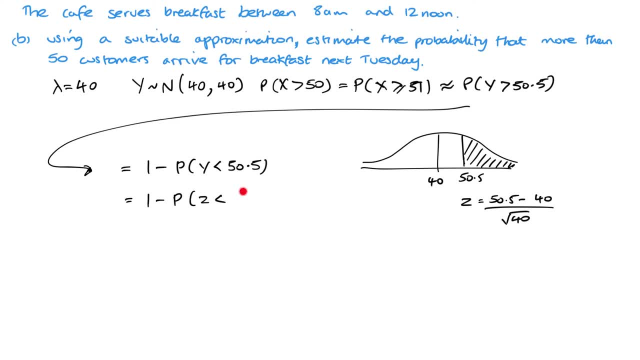 Obviously, if you were going to put it in the question, just put that straight in here, Or, like I'm going to do, is I just put that value in And this value is going to be 1.66, which I will pop there. 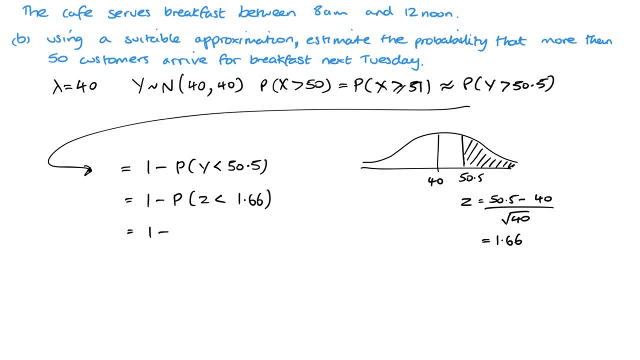 Okay, Now, if you're using your calculator, you can use your calculator to do the normal. And if you did, what I would say is use that full value of z. If you're going to use your calculator, If you're going to use the tables, you know, obviously use the rounded value. 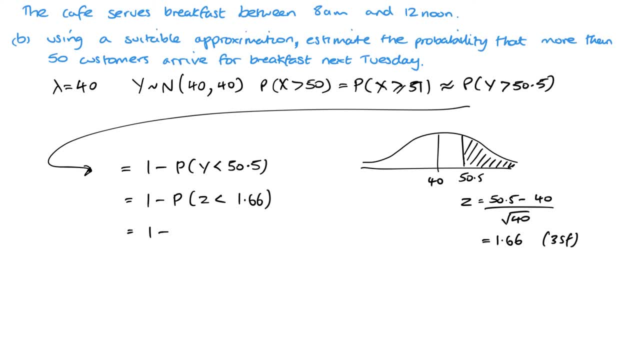 And you will be slightly off potentially but it shouldn't be anything to worry about And you'll notice in a lot of the mark schemes they'll give you like an answer from the tables and answer from the calculator. Here you can see my 1.66 gives me 0.9515.. 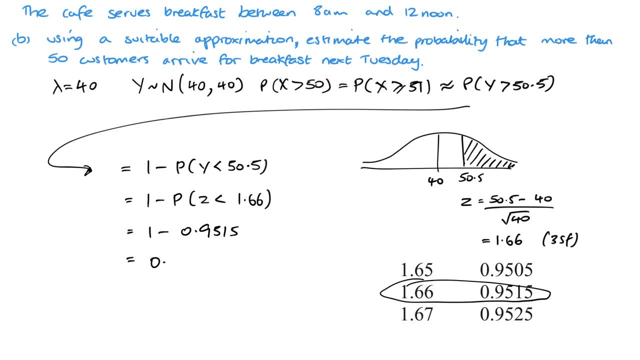 And 1 minus that is 0.485.. Oops, sorry, I missed out a 0 there. Get rid of this 0.485.. There we are, And that is a good enough answer there. That's from the tables. 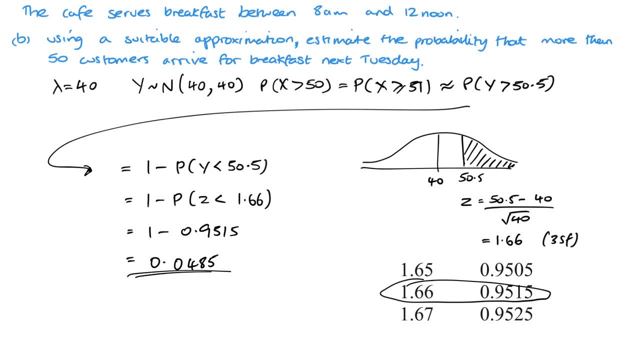 If, in this case, you used your calculator, you would have got 0.0484.. And you know a few others, So that's from the calculator. So if you do use that full value, you can see you will just get. 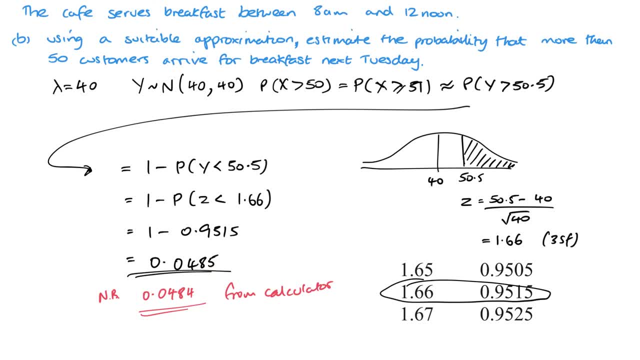 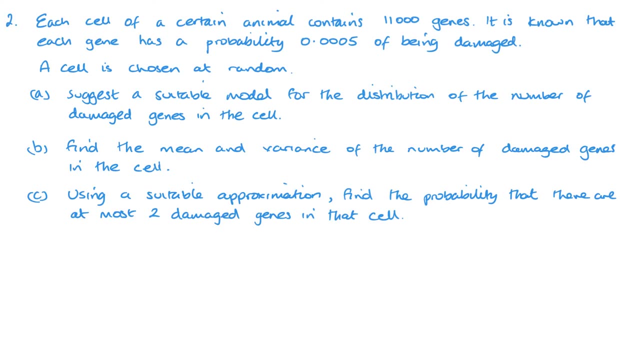 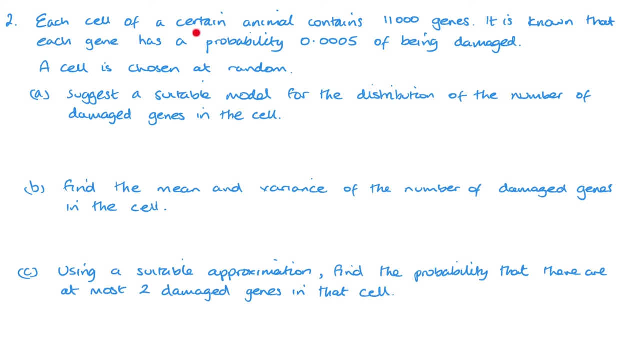 a slight difference there. Okay, it's 0.484.. And the next number is actually 4 as well. And that is this question done. Quite an easy question, this one. So, if we look at it in the beginning, each cell contains: 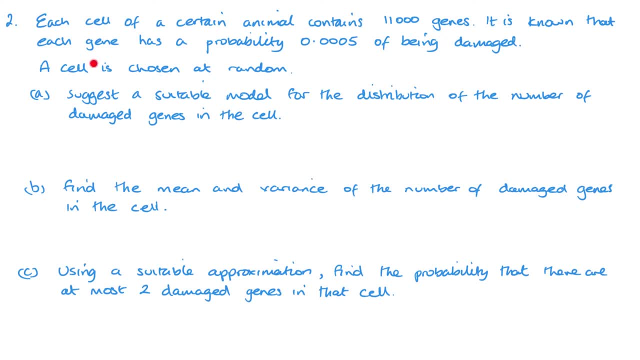 it's 11,000 genes And the probability is 0.0005 being damaged. So we've got N and P, haven't we? So you can see that this is clearly going to be binomial. So just a suitable model for the distribution. 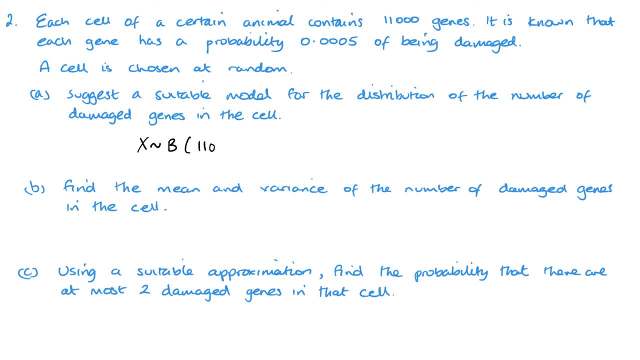 So there we have it. Binomial N is 11,000.. And P is 0.0005.. And job done there. Part B, then, is find the mean and variance, So our mean, or E of X, however you want to. you know, whichever kind of symbols you want to use here. 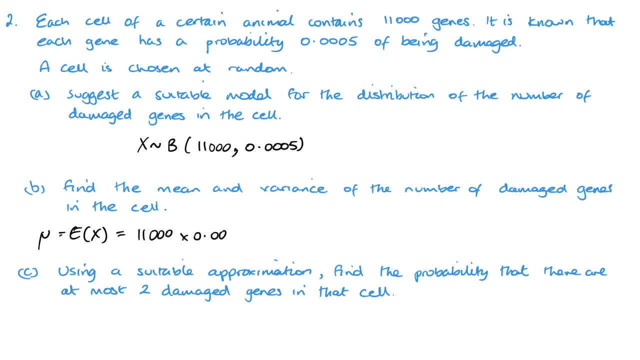 This is going to be 11,000 times 0.0005.. And that is 5.5.. And then we want our variance, don't we? So, again, it doesn't matter which, Whether you use a symbol or VAR, V-A-R-X. 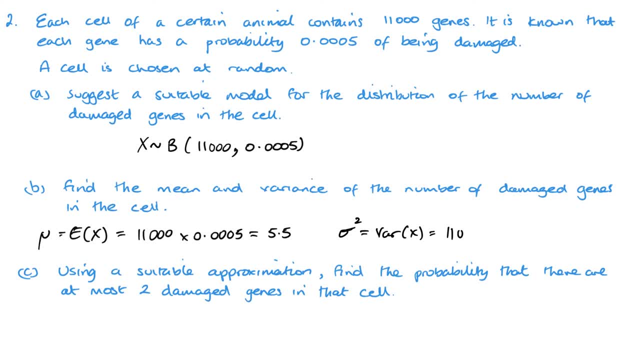 You know, totally up to you. So this is going to be N times P, times that, 1 minus P, isn't it, And that will give me 5.49725.. And I definitely would write this one out in full before kind of thinking about maybe rounding it off. 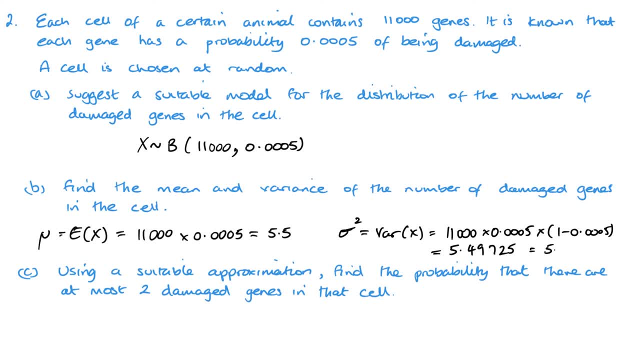 If I did round it off to three significant figures afterwards. so 5.50, I could. But I do need to make sure I have that one in full first, because you know if I just wrote 5.5, you know. 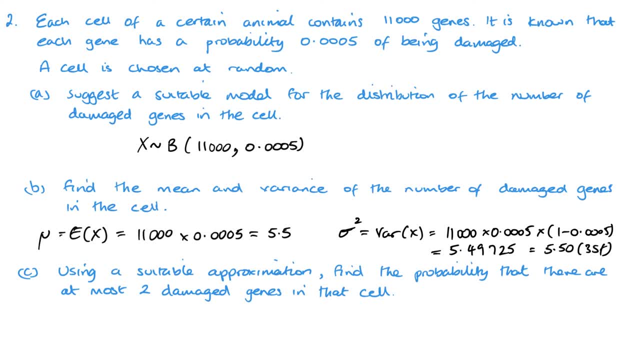 it is almost 5.5.. We do need to really show that. it is just slightly off, But it is pretty much 5.5.. So part C is about a suitable approximation. Now this is obviously binomial, as we said. 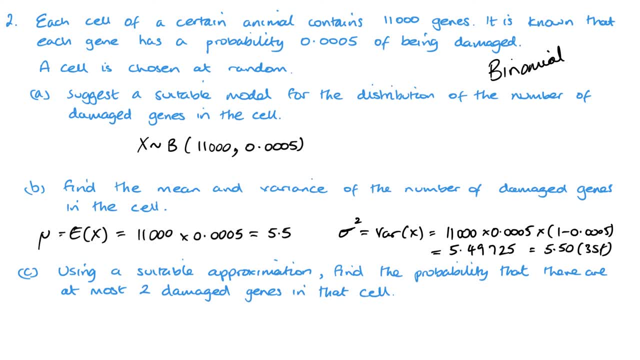 Which means binomial, can go to Poisson, or it can go to the normal approximation, can't it? In this case, I don't necessarily think about looking at whether you know it is obvious. You know we've got N is very large. 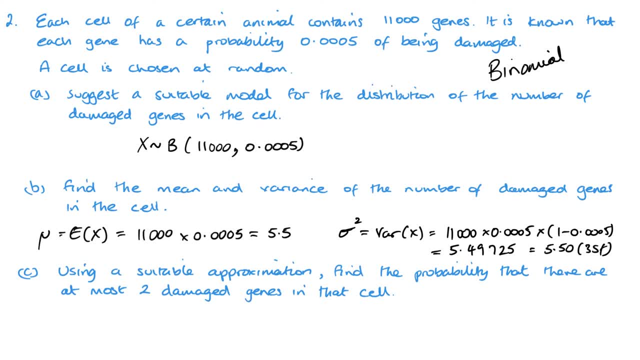 P is very small, isn't it Okay, which will imply a Poisson anyway. But from part B it's really obvious, isn't it? Part B, a mean and a variance are pretty much identical, And if your mean and variance are the same, that is one of the definitions for a Poisson distribution, isn't it? 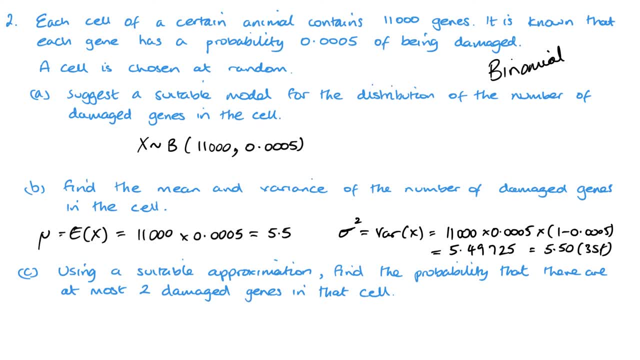 So you know there's two different ways there that you could get to Poisson, But it should be quite obvious for you. So y Poisson and this would be 5.5.. That is what they both round off to, But it's also Np, which is what lambda is. 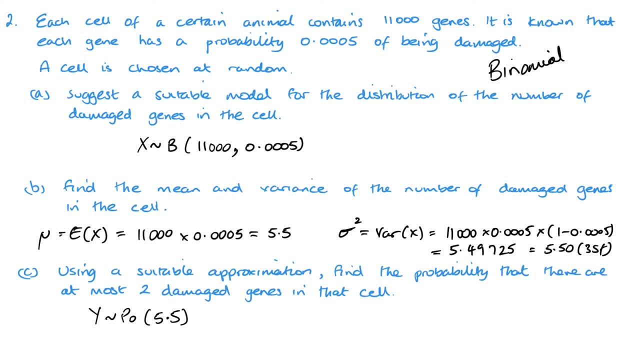 Now we're trying to find the probability that there are at most two damaged genes in that sequence, So at most two damaged genes. So we're looking at: y is less than or equal to 2. And 5.5 is a value that is in our tables. 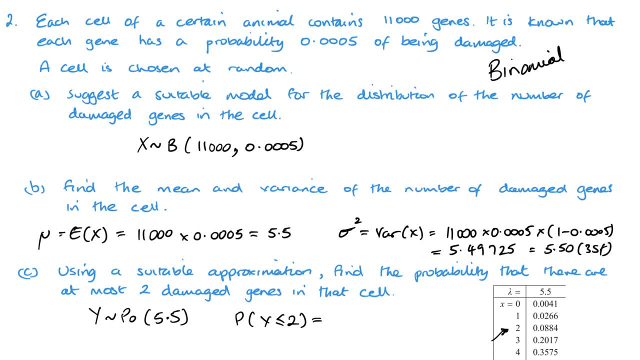 So let's bring those up, And here you can see it. So it's 0.0884.. Nice, straightforward question again. Okay, The difficulty really comes in that beginning Making sure you're comfortable. We know whether the question is binomial or Poisson. 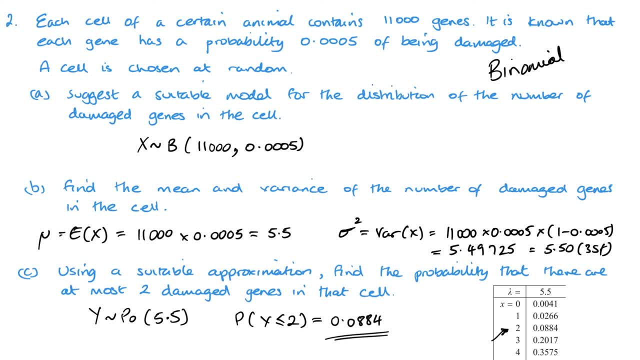 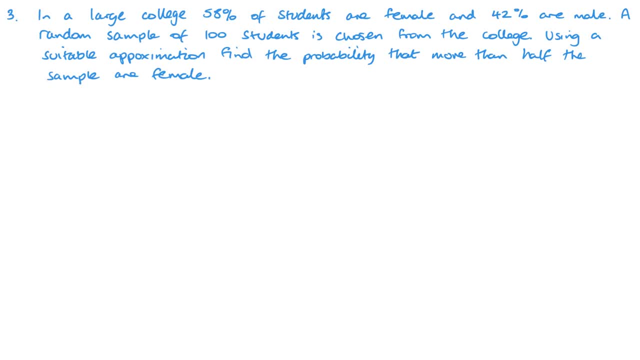 That is the key thing. Once you've got that down, then it starts to get much, much easier. So, looking at this question, we can see that in a large college, 58% of students are female, 42% are male. 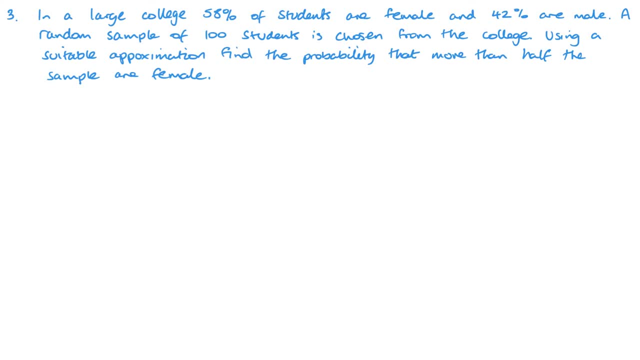 Random sample of 100 students is chosen. So we've got a fixed probability. We've got a fixed number of trials. Using a suitable approximation, find the probability that more than half the sample are female. So I think it should be quite obvious that this is initially a binomial. 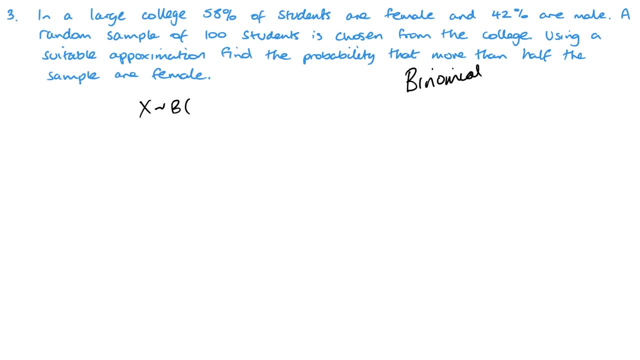 So we're looking initially like this: 100.. And we're dealing with female, So our percentage is going to be 0.58.. So that's where I'm starting. Obviously, now we need to kind of look at an approximation. So approximating this now. 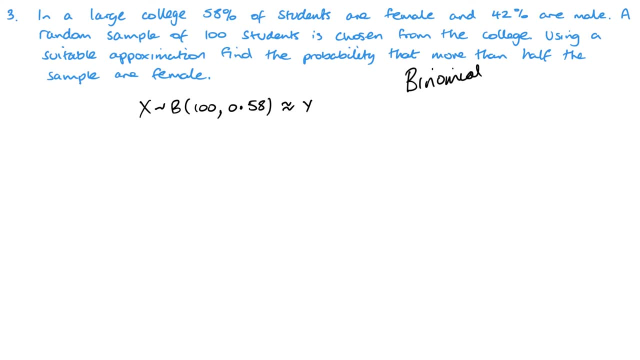 If you remember, it's going to be NP, So approximate, the normal Mean is NP. 100 times 0.58 is going to be 58. And then our variance is NP: NP multiplied by 1 minus P. So that would be 58 times 0.42, which gives me 24.36 exactly. 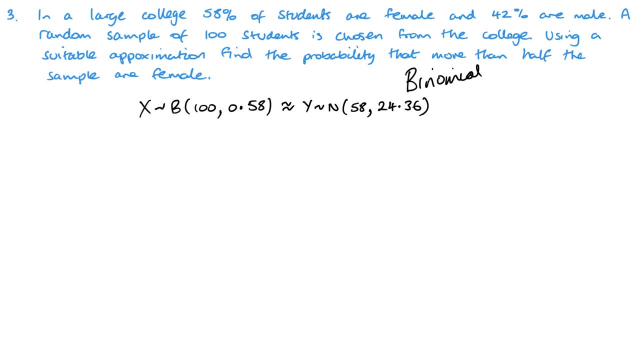 Now we want more than half, don't we? So we're looking at- let's make a little bit more room up here- Probability when Y is greater than 50. Which is obviously Y being greater than or equal to 51. I suppose, really, I should be saying this is X, shouldn't I? 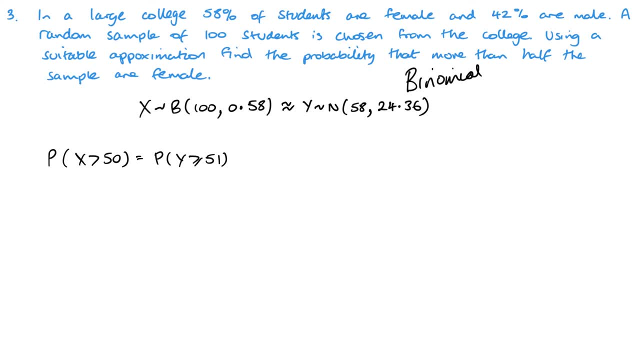 Let's do that as a change, Because that's what we're talking about. When I estimate this, that's when it's going to be turning into my Y And that's going to be greater than 50.5.. Okay, So don't forget that continuity. 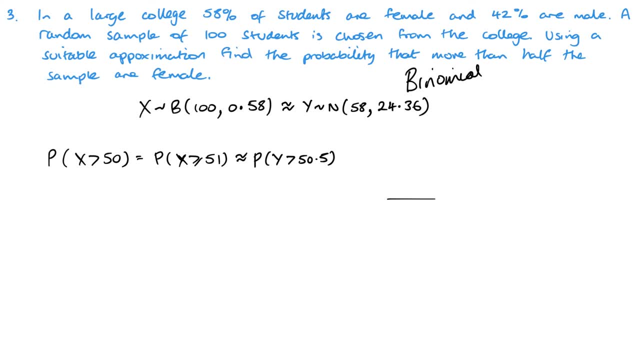 Don't forget that continuity correction. As usual. just going to do a very quick sketch. So if I think about it, the mean is 58, isn't it? And we are looking at greater than 50.5.. So that is what we're trying to find here. 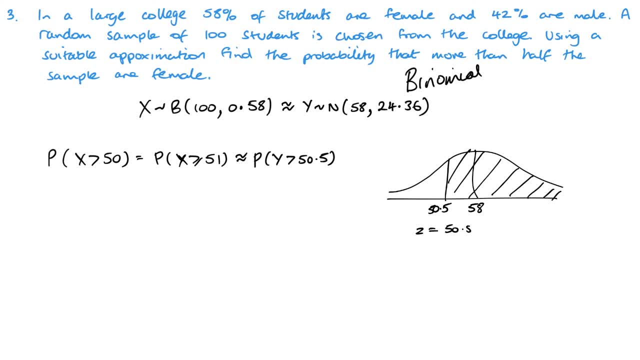 So first find my value of Z, So 50.5 minus 58 over the square root of 24.5.. 24.36.. And that gives me minus 1.52 to 3 significant figures And, as you know you know, flipping this around will give me this diagram with a positive 1.52 there. 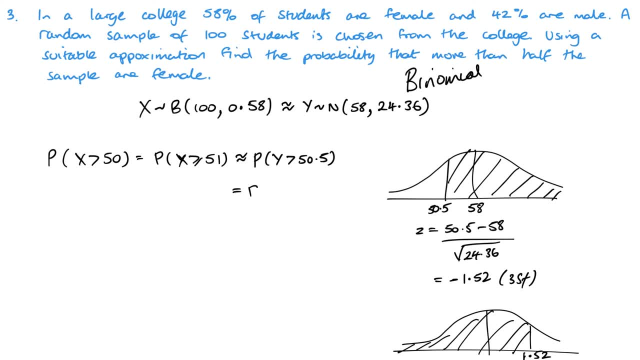 So that's what we are basically looking at, aren't we? So this is the same as Z being greater than minus 1.52.. Which is the same as Z being less than 1.52, but the positive 1.. And this, then, I can write up, or look up, I should say, in my tables. 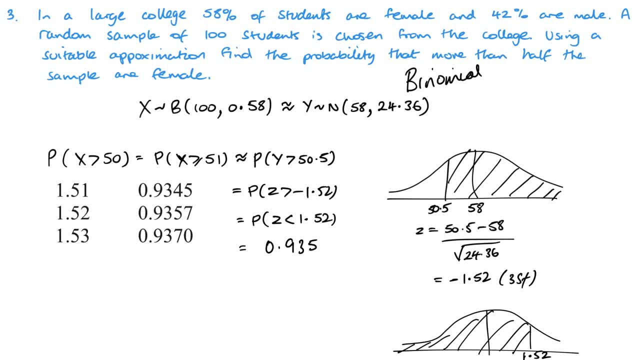 That gives me 0.9357.. And if you use the calculator, you would have got 0.9357 as well. 69, it was So in the calculator. same answer to four decimal places there. OK, Hopefully you found this video useful. 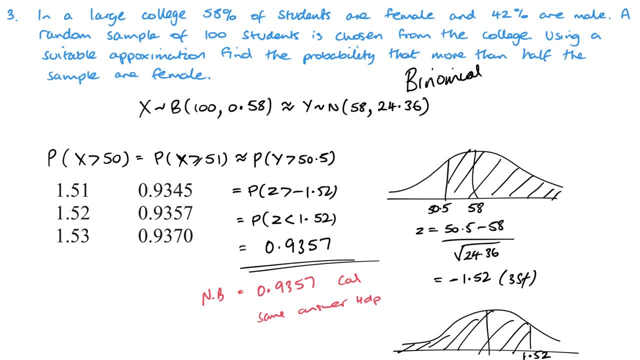 I know I've only done three questions. What I would suggest is try as many of these questions as you can And if you do find a past paper question that is particularly challenging, even if you manage to solve it, think this is particularly challenging, you know. 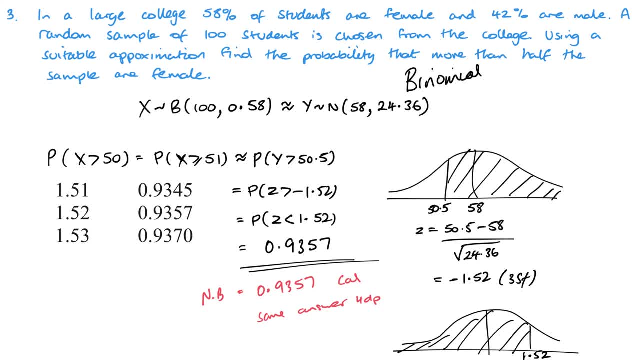 and you think it's worth me making a little video on or a few questions, then please send them through to me.